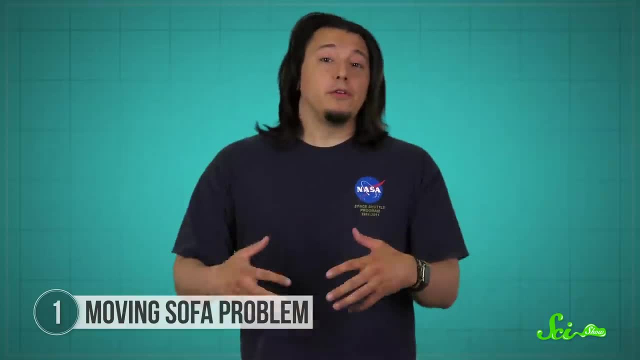 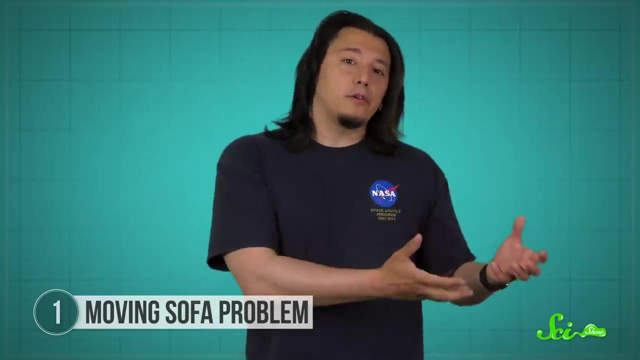 a specific number which the sofa area couldn't surpass, They concluded that either… Gerver's sofa could be the biggest possible sofa, or it's only a few percent smaller than the biggest possible sofa. So the solution might be near, but it requires all sofas to be tested. 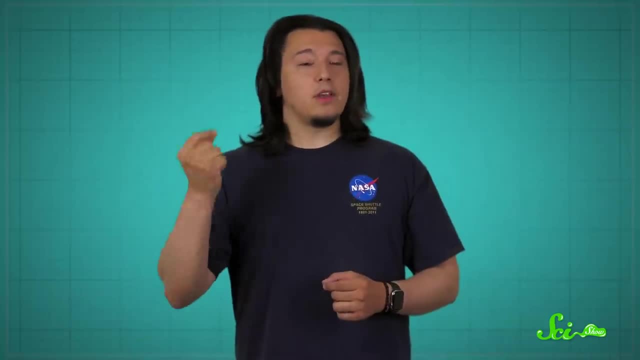 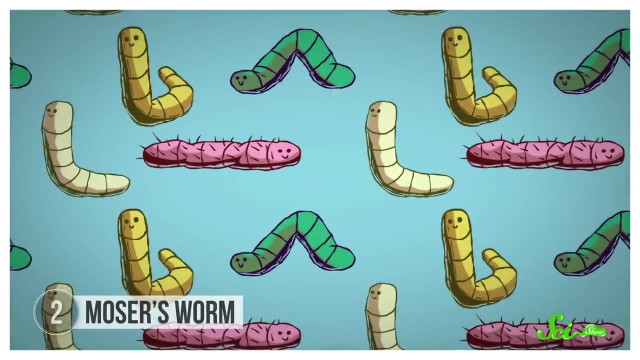 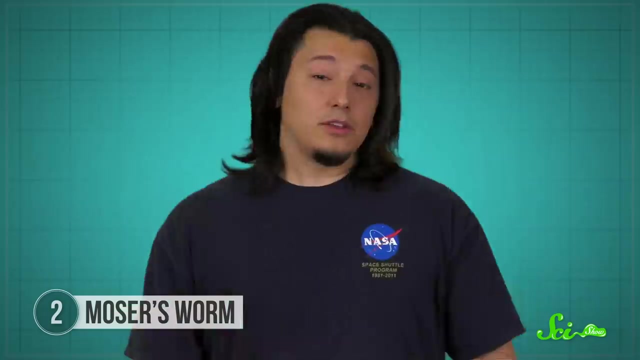 so the quest continues today. But the sofa problem wasn't the only problem Moser proposed. He also came up with a worm to go with it. We now call it Moser's Worm, or sometimes, lovingly, Mother Worm's Blanket. It involves a worm that wants to make a blanket that fully covers a sleeping baby worm. 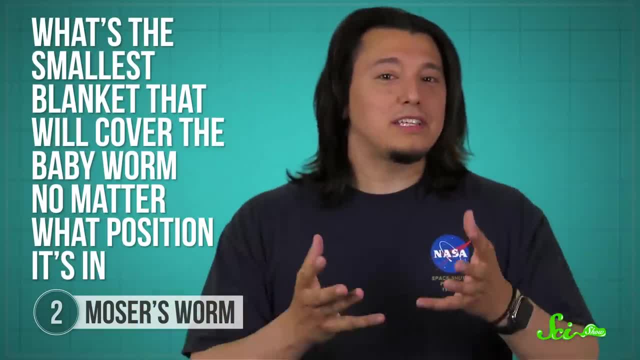 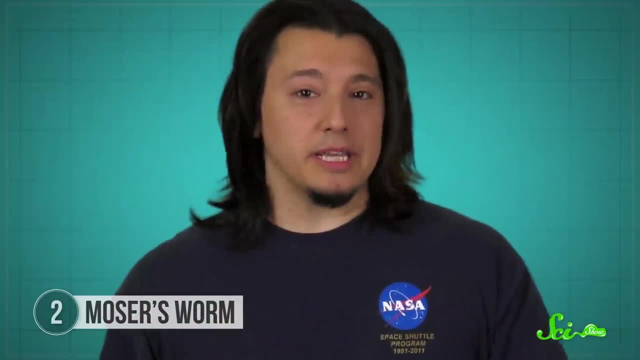 The question then is this: What's the smallest blanket that will cover the baby worm, no matter what position it's in? Well, say, baby worm doesn't move in their sleep. to make things easier, Clearly, a square blanket where each side is twice as long as baby worm would work. 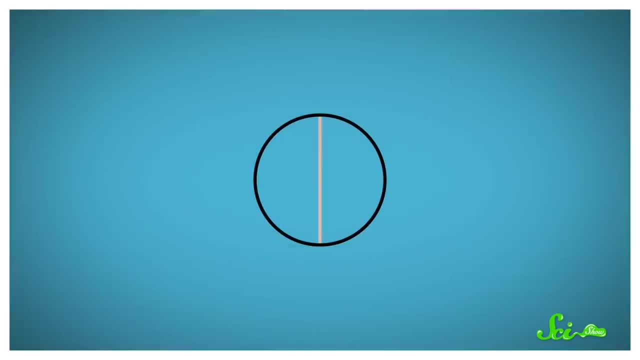 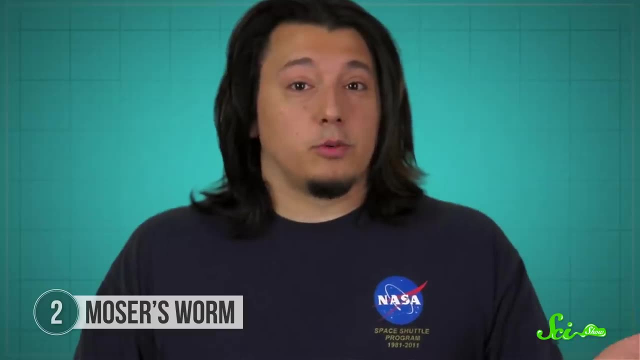 but you can go way smaller. Clipping the square corners to make a circle gives you a blanket that still works, but that blanket is only 79% of the square blanket's area. How much more can you cut off before it stops working? 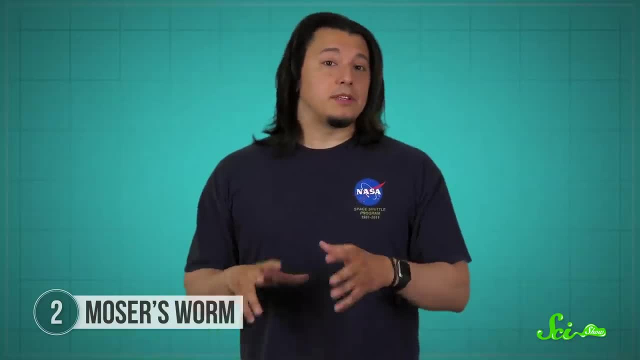 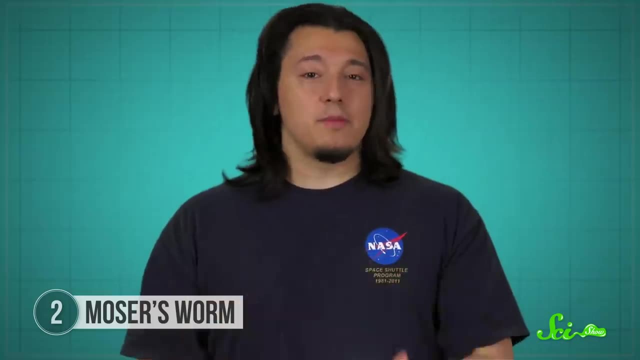 It turns out quite a bit Like with the sofa. When you have a sofa problem, finding a shape isn't the issue. Proving you've got the smallest one is. It's hard to check every shape one by one and even harder to prove it's the smallest one. 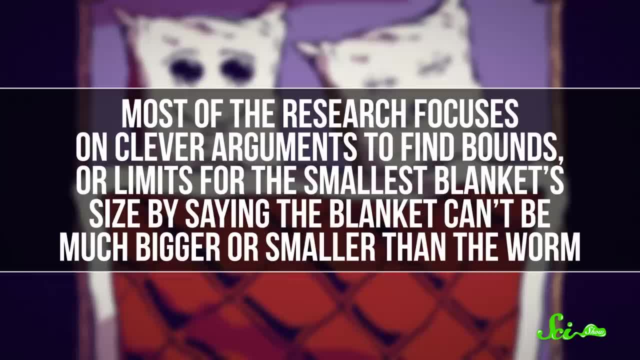 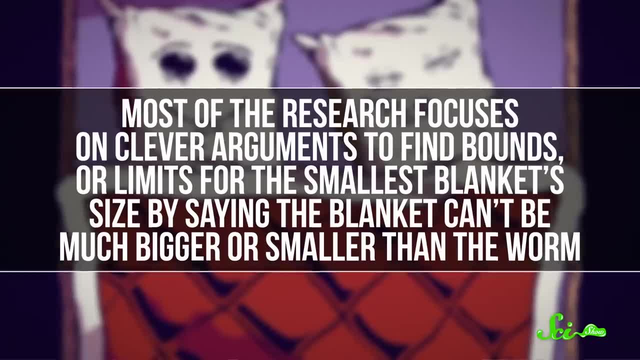 So most of the research focuses on clever arguments to find bounds or limits for the smallest blanket's size by saying: well, the blanket can't be much bigger or smaller than the worm. And researchers have actually come up with a bunch of clever proofs along those lines. 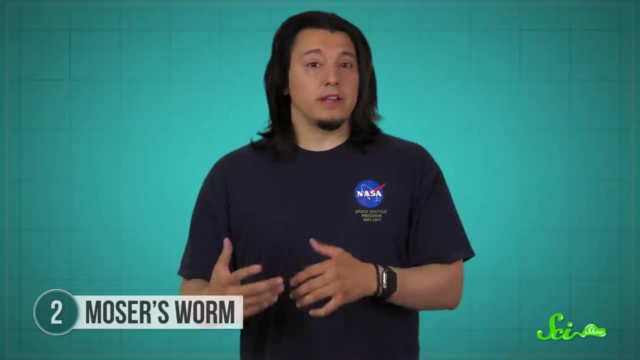 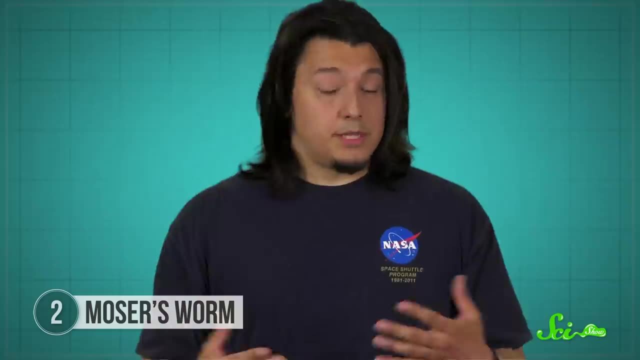 and narrowed down the limits quite a lot. Instead of needing a square blanket where each side is twice the worm's length, 6% as big can still cover the worm, no matter what position they're in. To be precise, it's now known that the smallest possible blanket is between 6 and 6.5% of the. 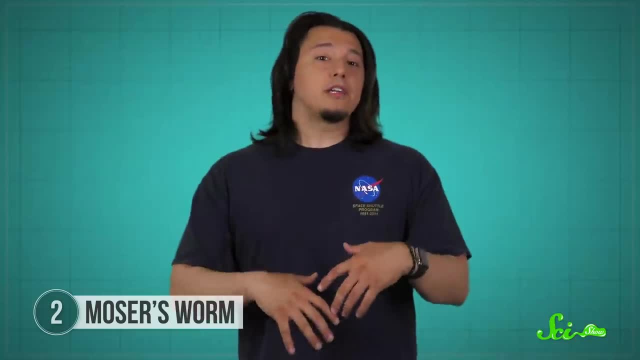 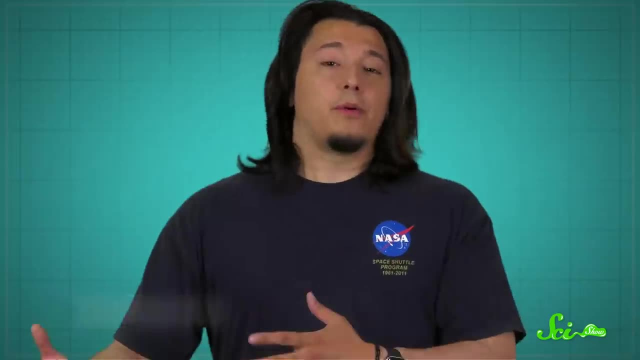 area of the original square blanket, And while researchers still don't know the actual size of the smallest possible blanket, whatever that shape ends up being will be saving Mother Worm a lot of knitting work. The worm problem turns out to have a surprising connection to another problem. that's a bit 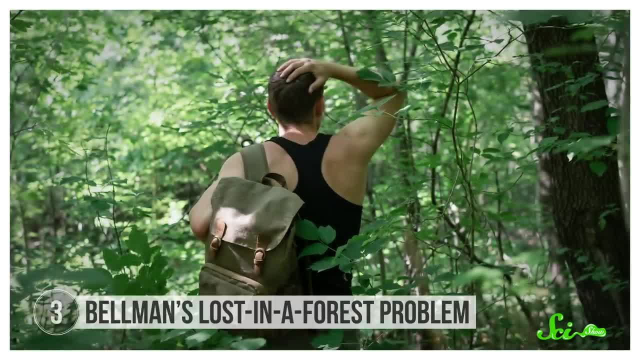 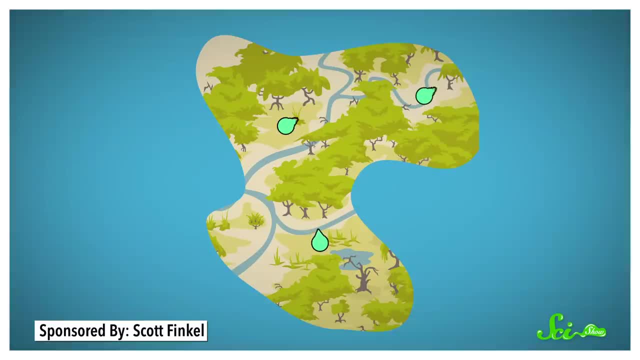 more survivalist-oriented. Imagine you're a hiker lost in a forest. You have a map with the size and shape of the forest but no landmarks, And on top of that you don't know which part you're in or which way you're facing. 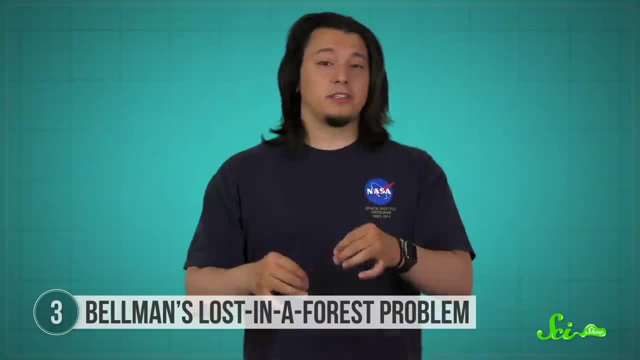 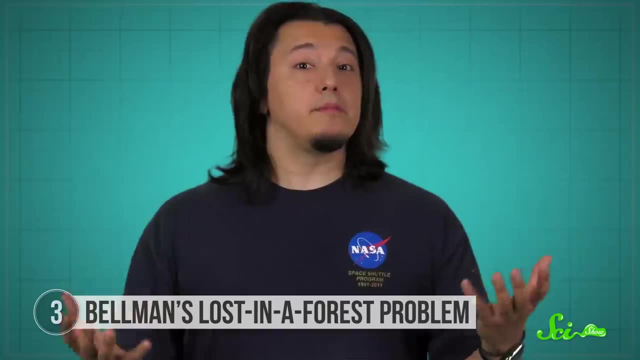 So how can you find the shortest path out of the forest? This is the lost-in-a-forest problem, which was first proposed in 1955.. In 2002, one researcher called it a million-buck problem, implying that it's secretly one. 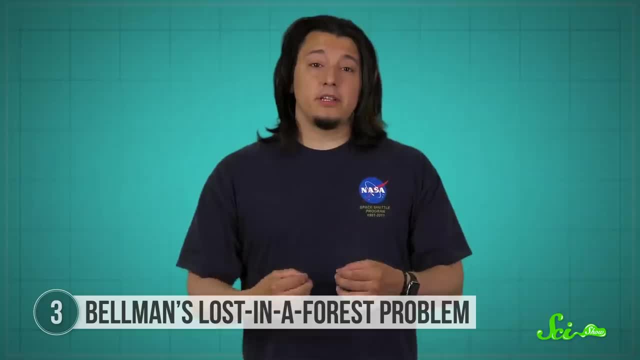 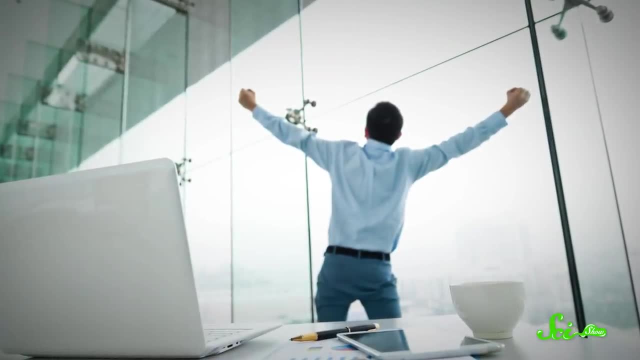 of the most important unsolved problems in math. He thought the techniques you would need to invent to solve the problem would be hugely useful in other areas of math as well. Sadly… the solutions are just as lost as the hiker when it comes to this problem. There aren't even many proposed solutions, let alone proven ones. The tough thing about this problem is that different shapes of forest turn out to be separate problems that need solving in different ways For circles as well as squares, pentagons and all regular polygons with more sides than. 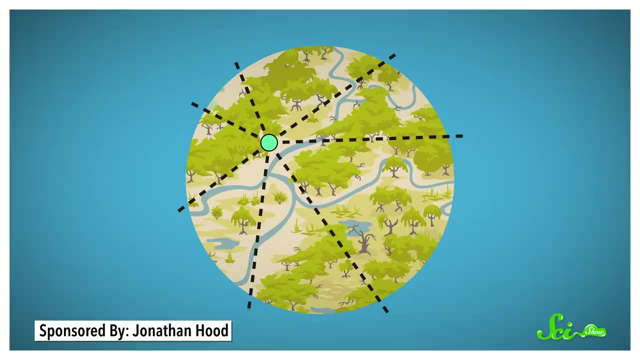 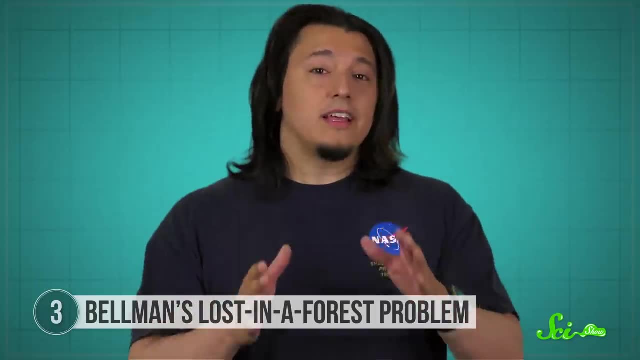 a triangle, it's been proven that a simple, straight line is the best path. That means that no matter where you are in those kinds of forests, walking in a straight line is always the fastest way to escape. But a straight line isn't always the best option. 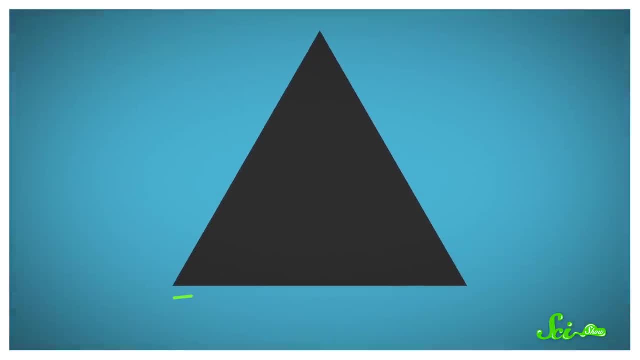 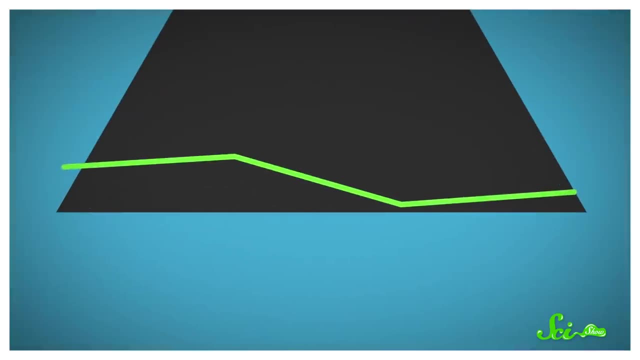 It depends on the shape. For equilateral triangles, it's known that a certain kind of zigzag pattern is the best path to try. That's because it's been proven that there's a zigzag line that doesn't fit inside the triangle, no matter how hard you try to slot it in, and that zigzag is shorter than the. 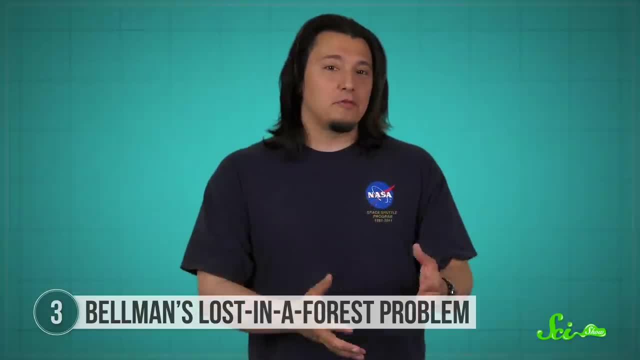 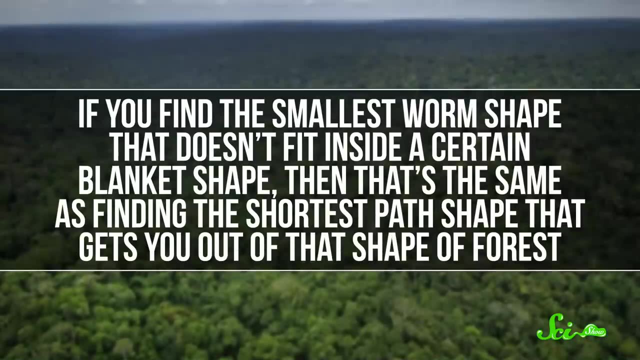 triangle's sides. So working on the problem can be tough. But progress in this problem can also be used in the worm problem, because the two are kind of inverses of each other. If you find the smallest worm shape that doesn't fit inside a certain blanket shape, then you're. 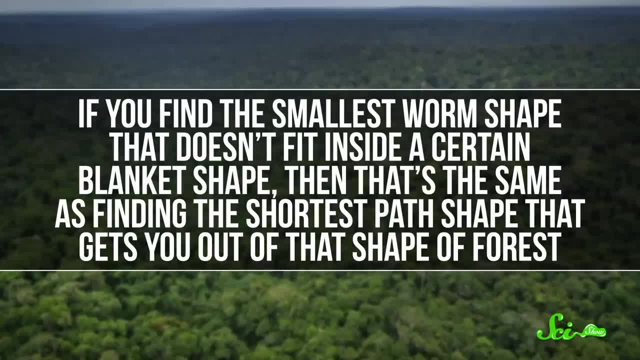 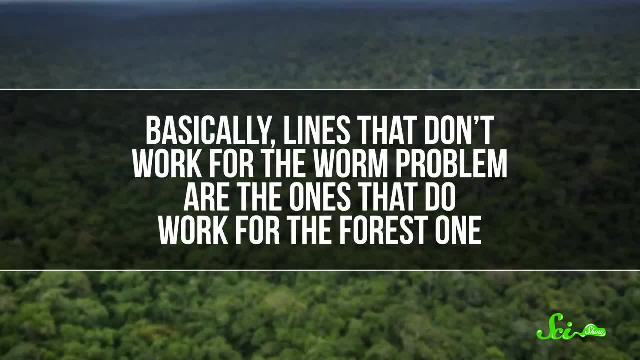 done, Then that's the same as finding the shortest path shape that gets you out of that shape of forest. Basically, lines that don't work for the worm problem are the ones that do work for the forest one. Some recent work has hinted that maybe there's a simpler way to check if a certain type of 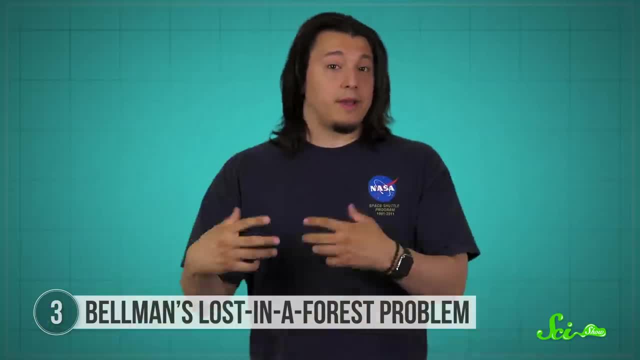 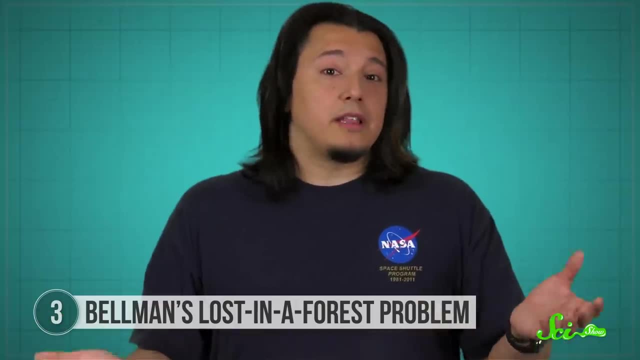 path is the shortest possible for a particular shape of forest. And making paths easier to check means that researchers might be able to use computers to check a bunch of paths really quickly, So researchers may not be lost in the woods for too much longer. Moving away from geometry, 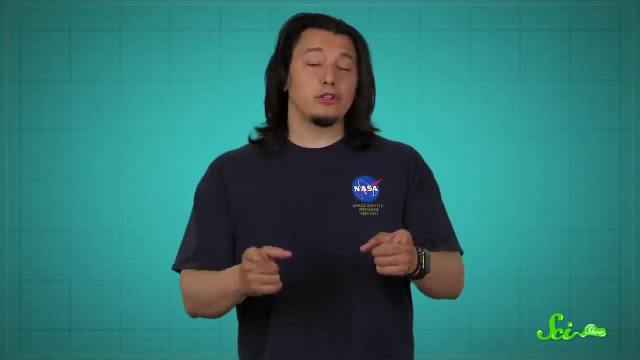 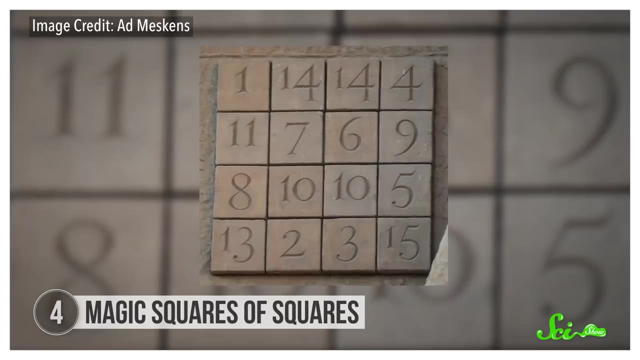 Another neat unsolved mystery is about numbers, and it's actually a problem you can try to solve right now. It involves magic squares, which are grids of different numbers where every row, column and diagonal adds up to the same number. This is not a new problem. 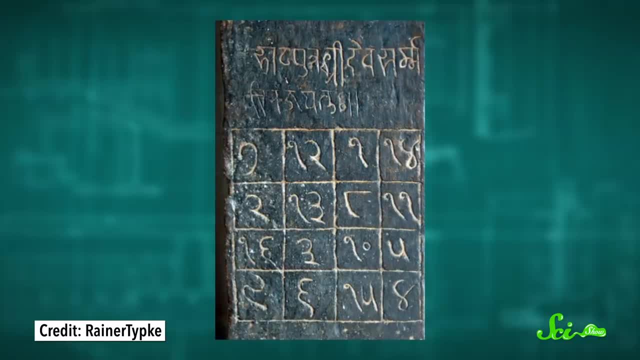 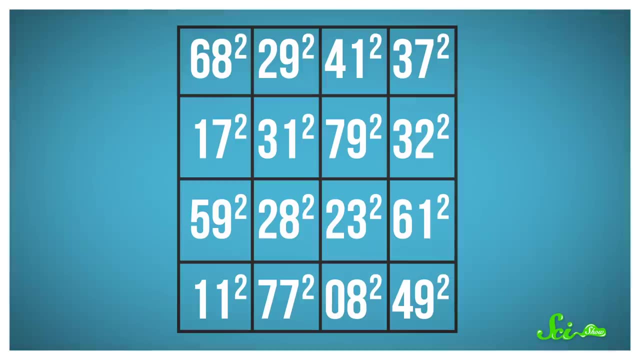 It's been played with for thousands of years, from ancient China to medieval India, to 18th century Europe. The unsolved problem is about magic squares of squares. Magic squares made only of square numbers, which are numbers you get from multiplying a number by itself. 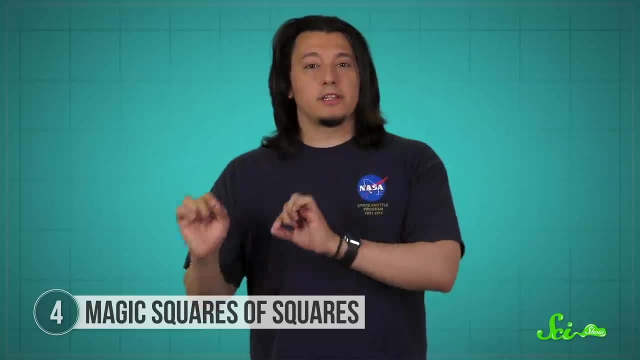 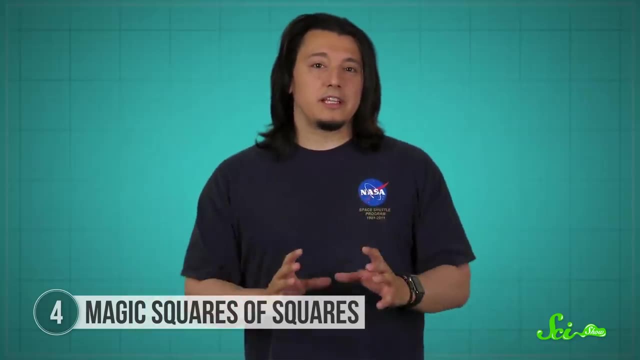 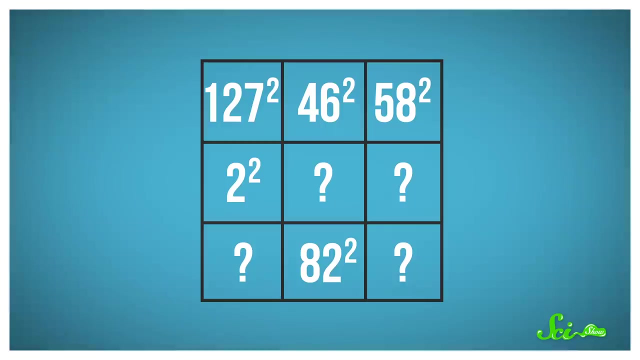 The most famous and unsolved one is the three-by-three magic square of squares, made famous in 1996 by legendary puzzle maker Martin Gardner in one of his Scientific American columns. Again, this puzzle sounds simple, right? All you need to do is write down the correct combination of nine numbers and you've solved. 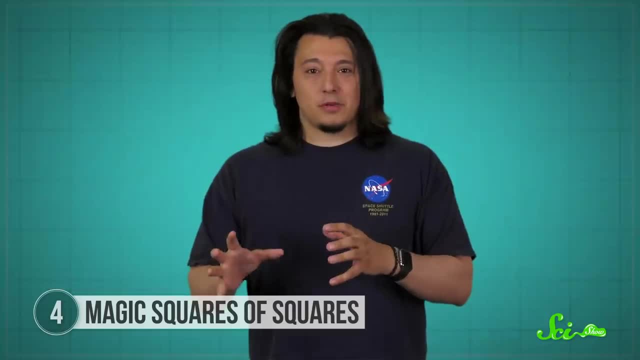 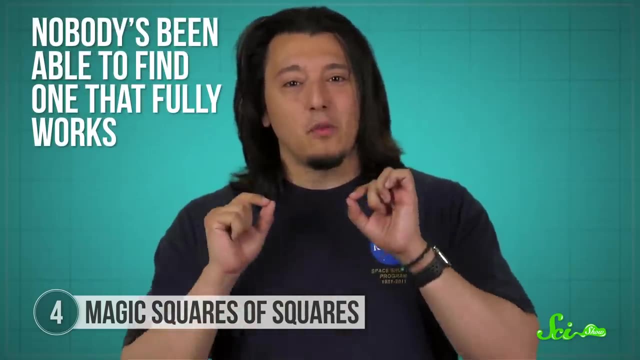 it Like an extreme Sudoku. There have been a lot of near-misses, Magic squares, where two of the numbers aren't squares, or where one of the columns doesn't work right, or some numbers repeat, But nobody's been able to find one that fully works. 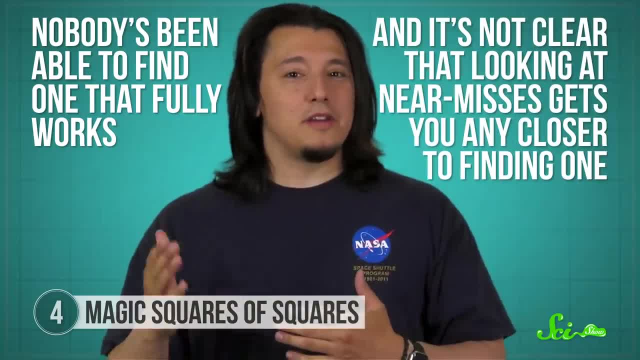 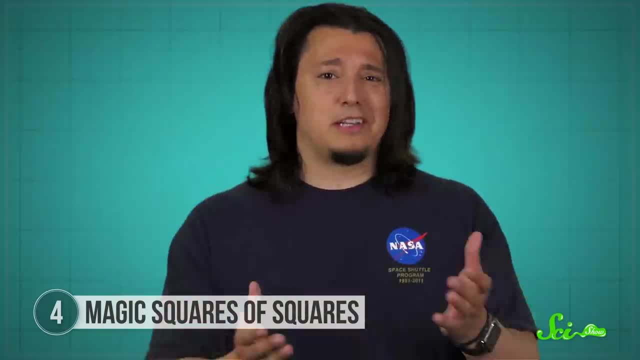 And that's why we're here today. And it's not clear that looking at near-misses gets you any closer to finding one, And maybe there simply isn't one that fully works. But if that's the case, why? Why does it work for all those other examples, but not here? 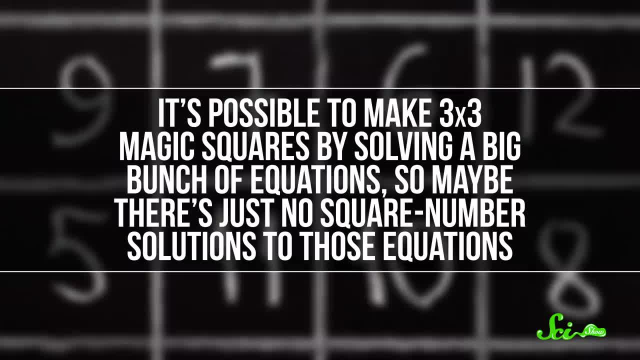 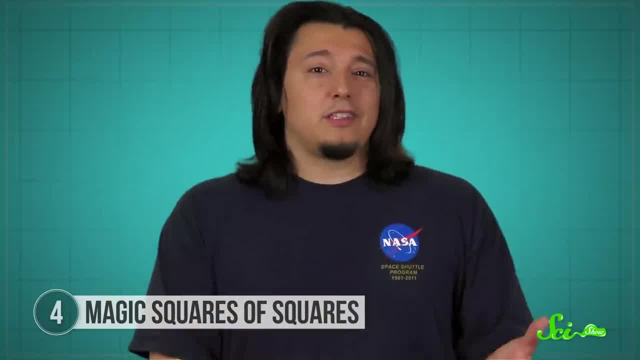 It's possible to make three-by-three magic squares by solving a big bunch of equations. So maybe there's just no square-number solutions to those equations, though no one's been able to prove that. That feels a bit unsatisfying as an answer. 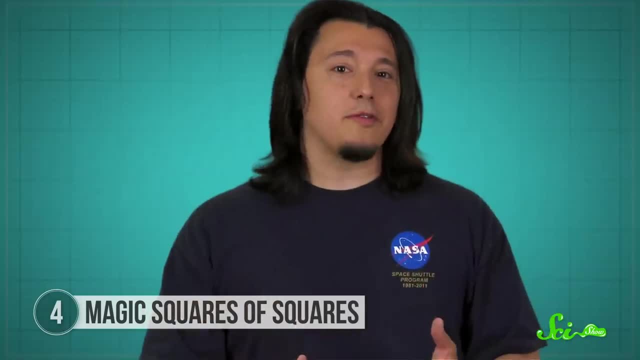 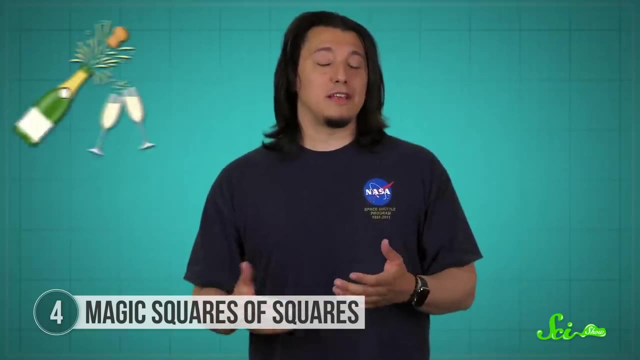 So many people, mostly hobbyists, still hope there's a solution out there and spend their time searching for it Until someone proves it can't be done. In fact, one person has offered a prize of a thousand euros and a bottle of champagne. 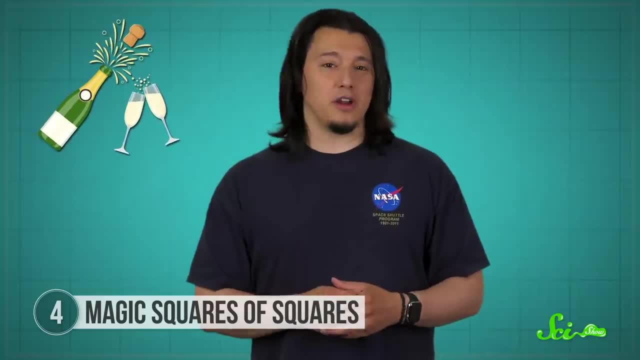 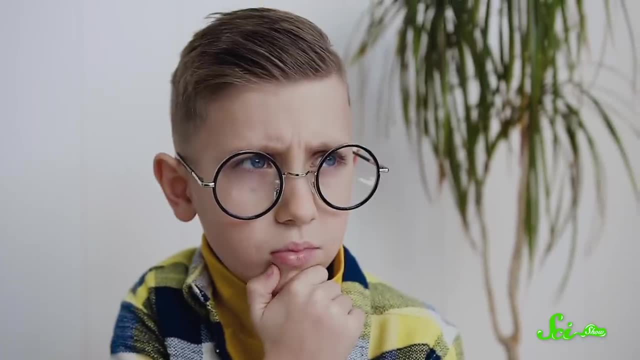 to anyone who finds a three-by-three magic square of nine unique square numbers. Not quite a million dollars, but not bad either. And the really cool part is that you don't need a math degree to look for a square that works. Anyone can just go out there and start playing around with numbers, making this a neat introduction. 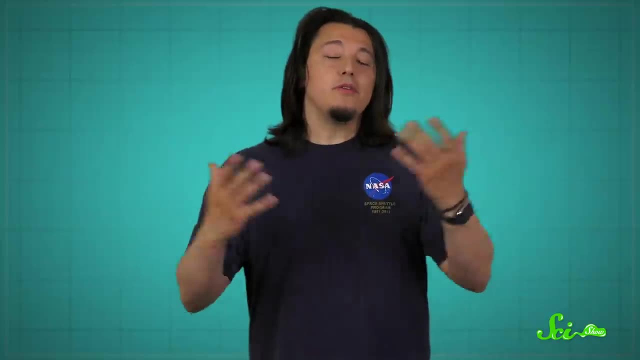 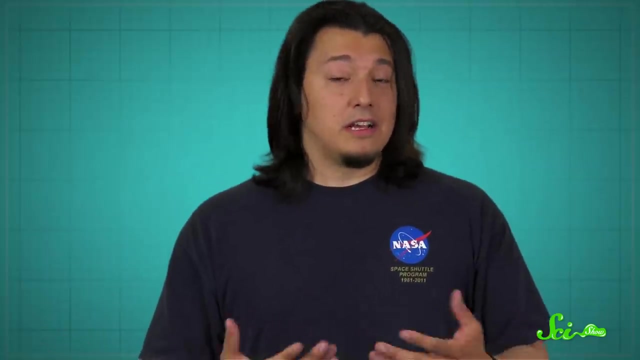 to the joy of recreational math In general. the beauty and fun of math is precisely in asking and answering those kinds of puzzles. Problems like these end up being surprisingly useful in the real world. But it's just as worthwhile to play around with these weird problems for their own sake. 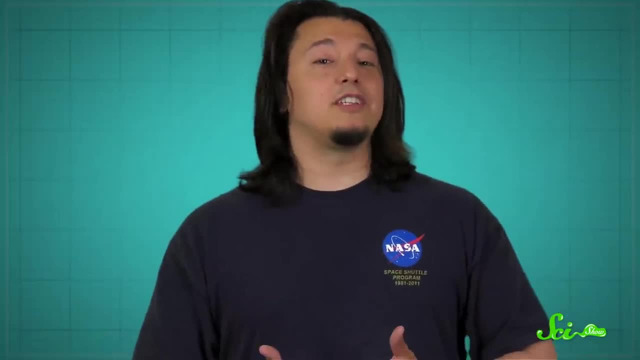 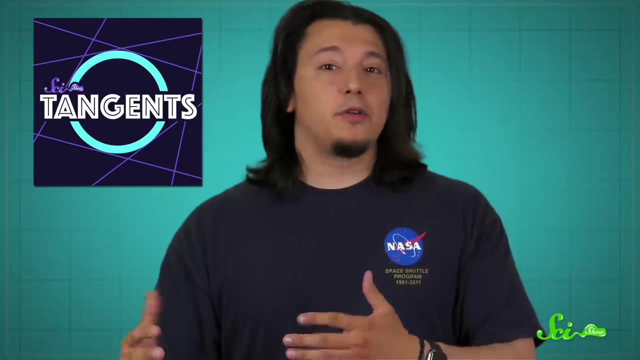 If you like these math problems then I bet you'll like a podcast full of tangents. SciShow Tangents is a podcast where the fun people of SciShow get together for a lightly competitive knowledge showcase. Every episode they rack up points for teaching the others and everyone listening at home. 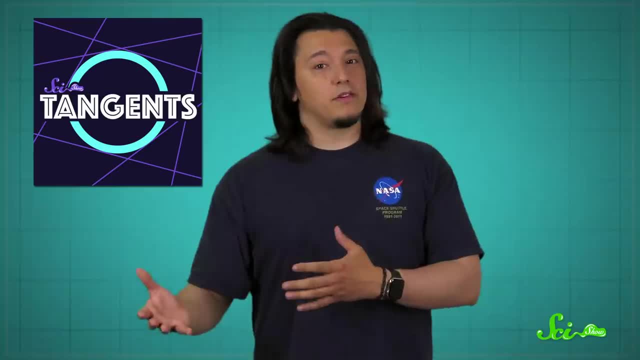 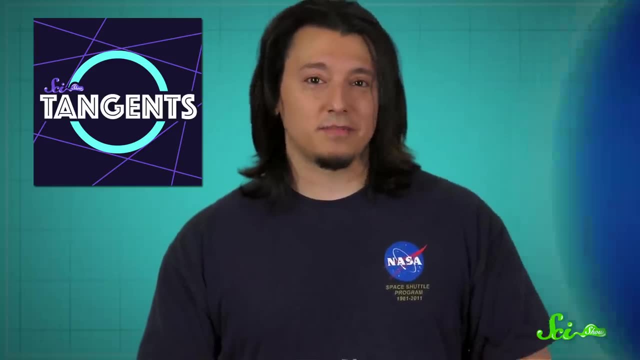 the most mind-blowing science facts related to the week's theme. If you love science, laughing and light-hearted nerdy competitions, you should check it out. You can find SciShow Tangents anywhere you get your podcasts.